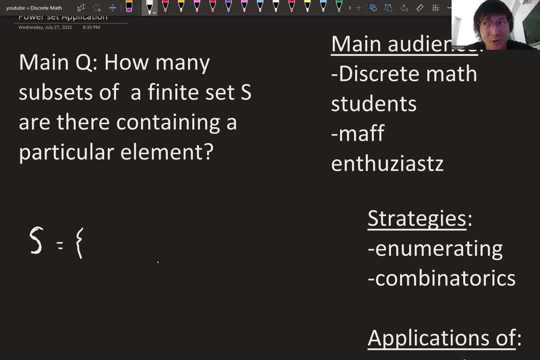 let me say that the elements. they're going to look like this. I was going to use lowercase s, but my handwriting is crap So let me change it to x, right? So let's say that the elements of s say: we don't know the number, but we know it's finite, So it's fixed, right So? 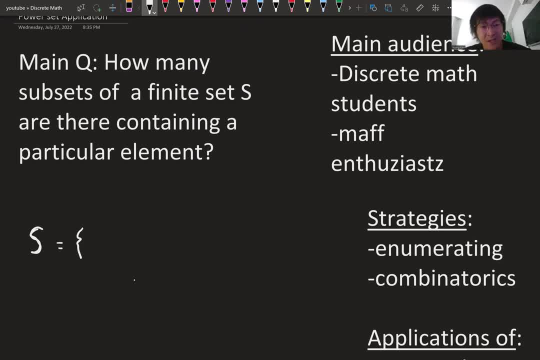 So then use an arbitrary letter to represent this right. So here I'm going to use n. So then that means that say that there's x1, x2, comma, comma, dot, xn and elements where for some n in the natural numbers. okay. 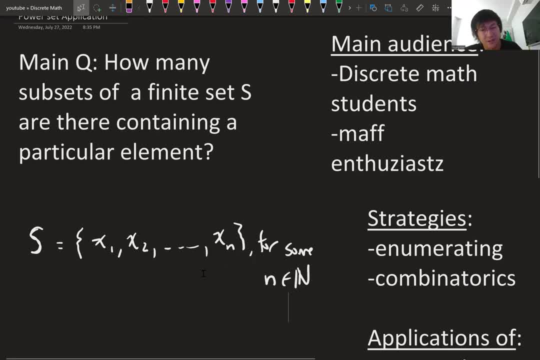 So this is just a fancy way of saying that this is a positive integer right And it's just counting this how many this is right. So there are n elements in here And just a little side note. this is a kind of little rant in itself. 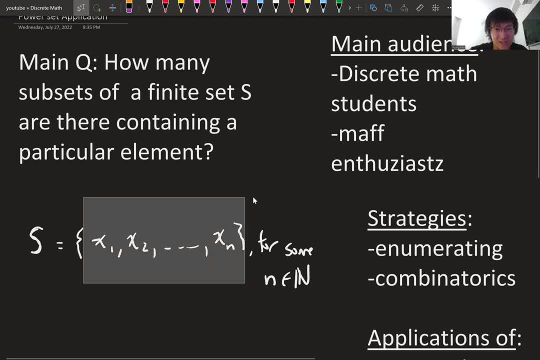 but when you see this right, the way that I listed this, it kind of implicitly assumes that n is greater than 2, because I wrote x1,, x2, comma, dot, dot, dot, dot, dot xn. But usually there is no. 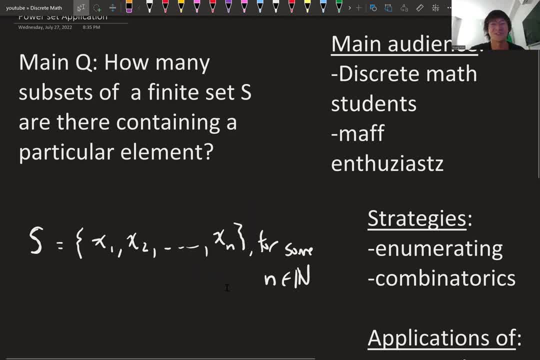 like universal agreement on this. So when you see something like this, like just assume that n could be 1, could be a single element in this set, right, But people need to talk about this more. I think there are some people that really get into the details. 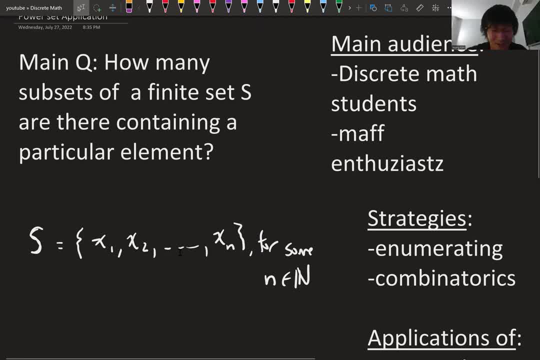 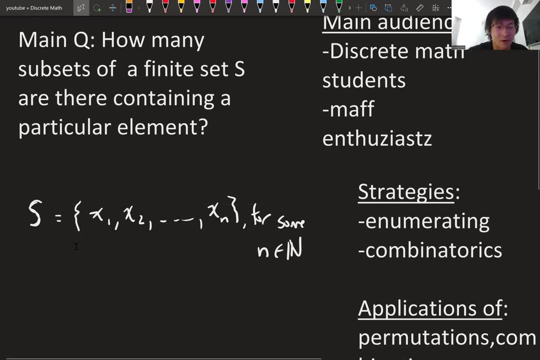 in their textbooks and stuff, and that's really good. But yeah, all right. So, anyways, so you have an n element set and then you want to see how many subsets of a finite set S are here, right? So this has something to do with the power set. all right, 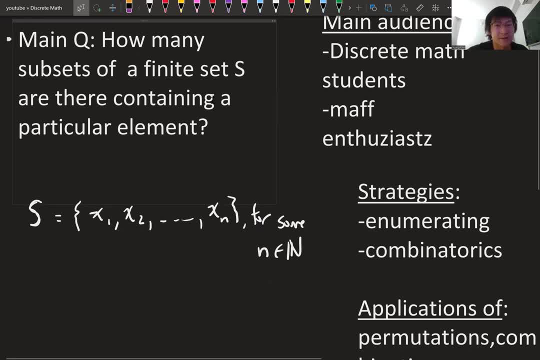 But here let's say that you are trying to create sets that are containing a particular element in here, right? So here I'm going to choose. let me just choose one. It really doesn't matter, right? So I could pick x2, x, sub 1 or something. 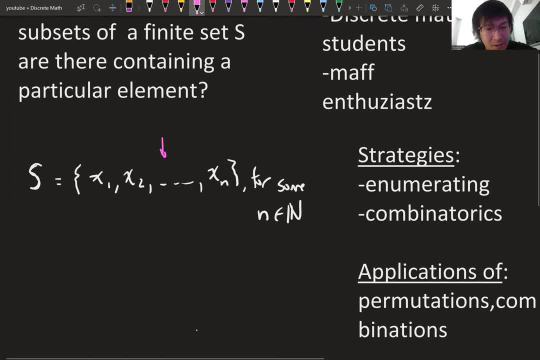 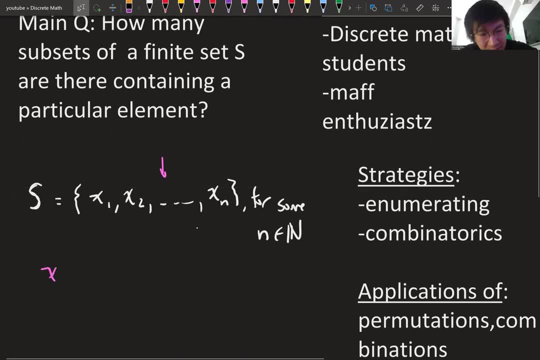 But in general we could just say: choose x, say that the element, this particular element, right, This particular element is x sub j. okay, X sub j for some, j for some j in between this right. So it's got to be 1,, 2, dot, dot, dot, dot n. okay. 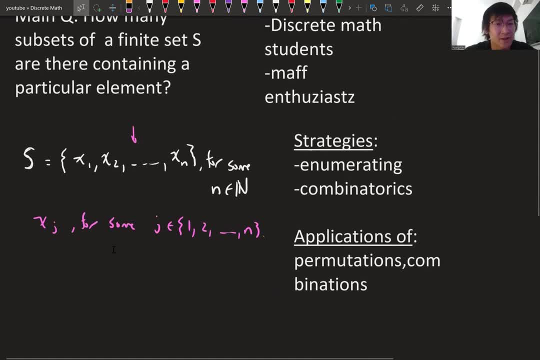 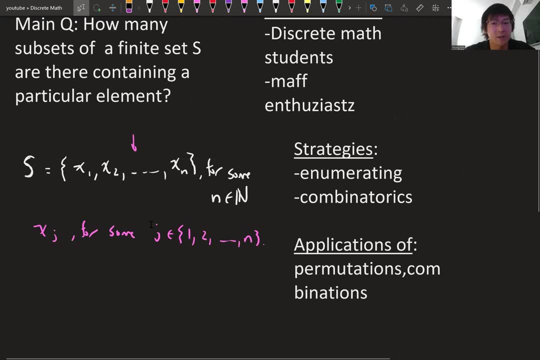 Great, So to find the number of subsets containing x, sub j. you can solve this two ways. I mean, there are at least two ways right. One by enumerating the set. So, given that you know, like, if you actually have like, for example, 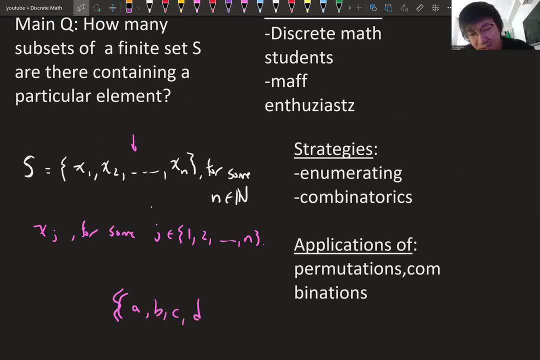 if I said like a, b, c, d, all right, So it's a four element set, And say that x sub j, here is e, then you choose this and do it. But then it gets really really hairy. you know if your set is really really big right. 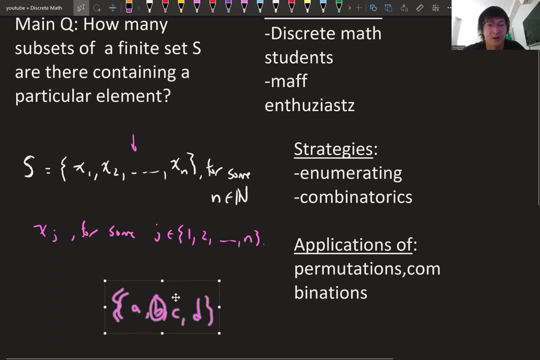 So here, this is taking care of the arbitrary case. All right, So then, if this doesn't work, then this is what you should go for. It's combinatorics, And you will see how this thing is so useful, right. 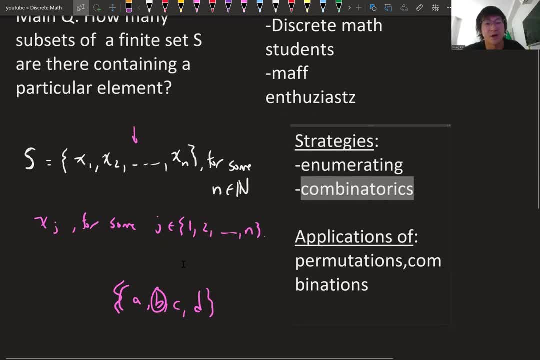 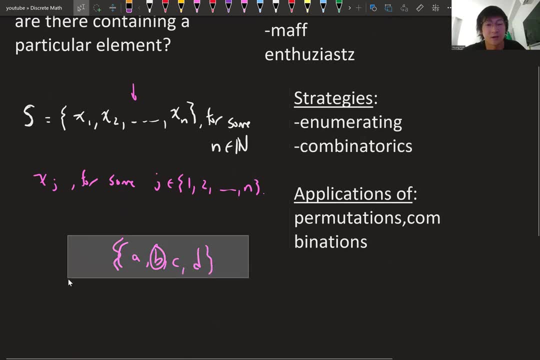 Like when I'm going to count this right How we do this, And then after we'll do an example, like a concrete example to show that this is okay. okay, Yeah, So here x sub j. so it's this: 1, 2, dot, dot, dot, dot n. okay. 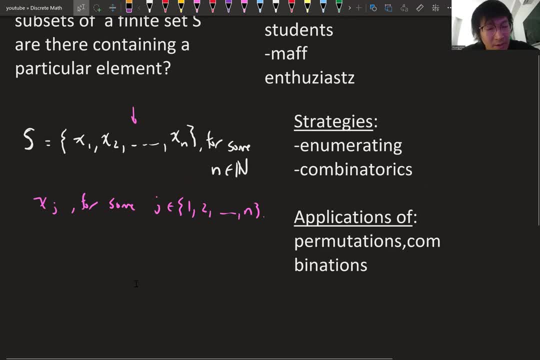 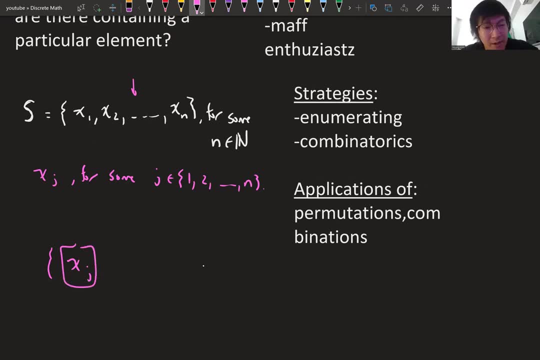 So here it's got to contain this x, sub j, So this means that your subsets have to look something like this: right, At the bare minimum. okay, Right, And then there could be other stuff in here, and this stuff in yellow would appear in here, right? 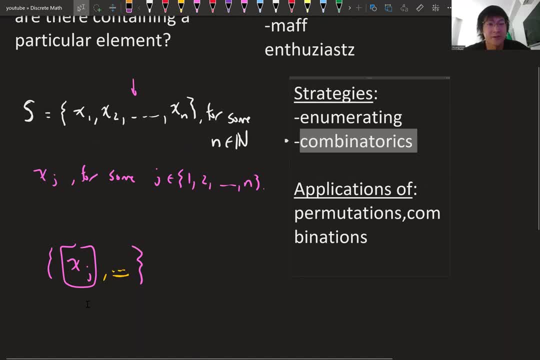 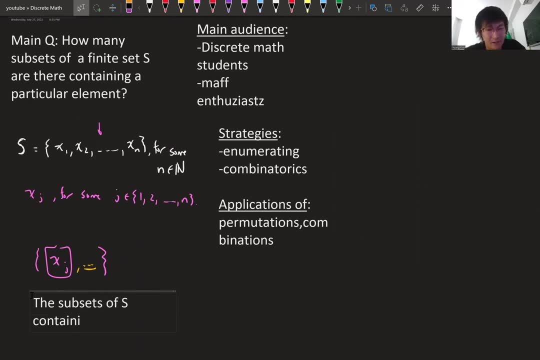 So this is where the combinatorics stuff will come in. okay, So you could say: the subsets of s containing x, x sub j will, oh, shoot, will have x sub j, necessarily Will have x sub j, and you could pair it with. you could choose 1 extra, 1 extra element here. 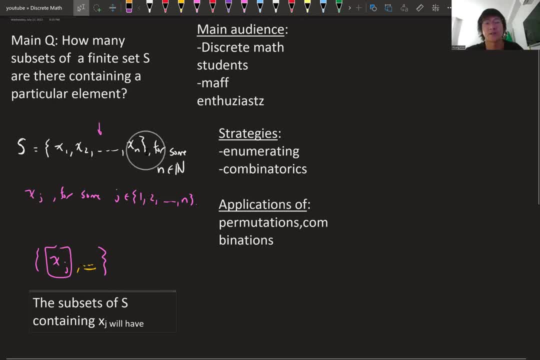 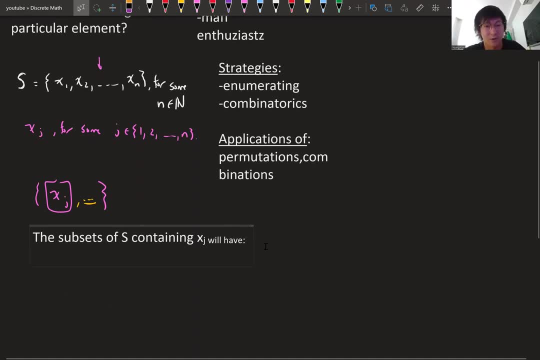 or 2 extra, 3 extra, all the way to n minus 1, because you already picked this one right. So the subsets of s containing x sub j will have. okay, exactly, so here's by case. so this is the numeric. I'm going to enumerate this by cases exactly. 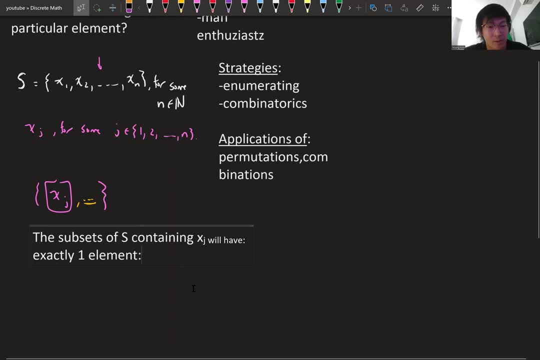 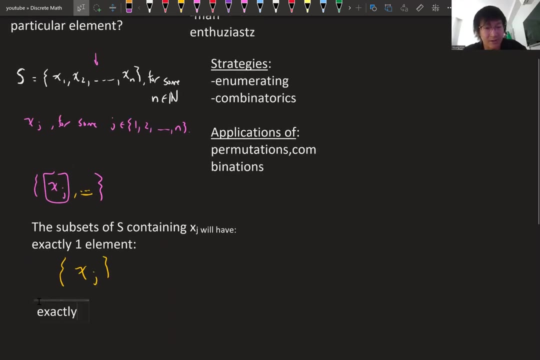 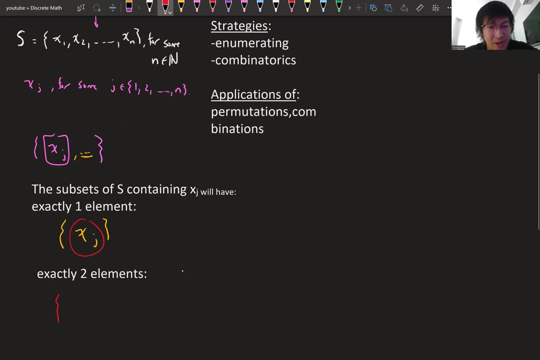 one element right, so that's just the singleton right, the singleton with or the single set with, just x of j, right? that's the only way you can do this, and then you do this again. but here, exactly two elements right, and we necessarily, we necessarily have to have this, so we have to have. 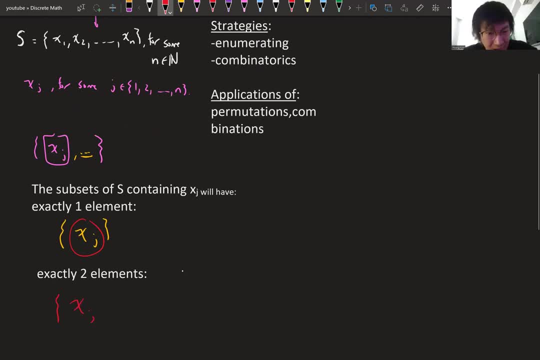 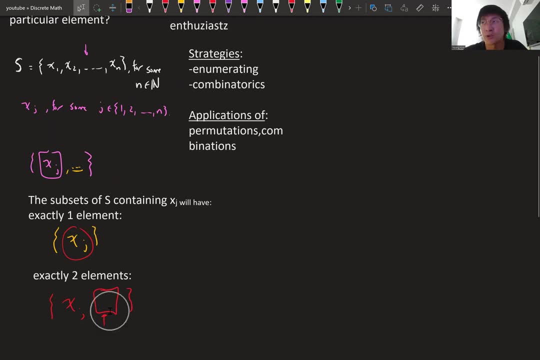 that redundant what I just said. but yeah, so you have to have that. and then you have to pick another element from your set, from this set that is not this. so you have to ask yourself: how many choices do you have? well, if I'm telling you that there are n elements in this set, then that means that 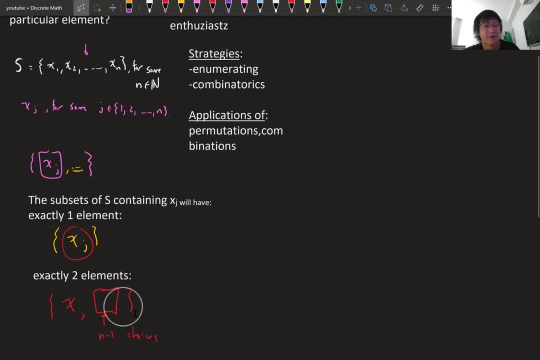 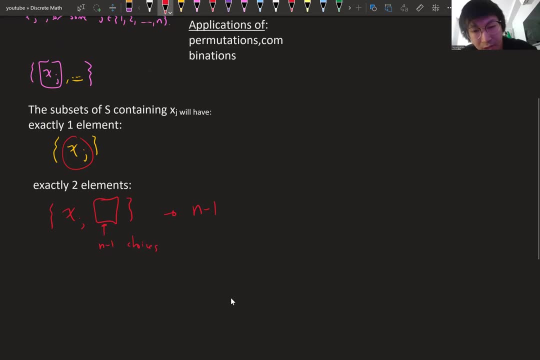 there are n minus one choices, okay, so then this thing: there will be uh, n minus n minus one of these, n minus one of these sets, okay, so then, uh repeat the argument again for exactly three sets, three elements containing. 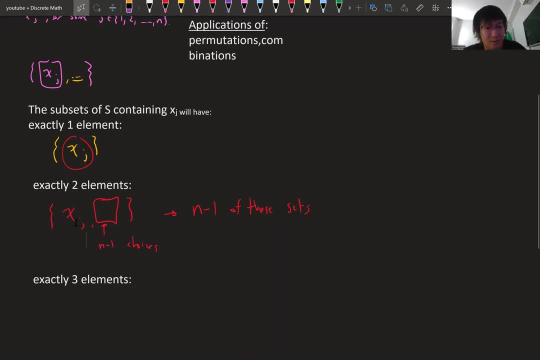 uh x of. I should put a comma here- uh x of j. well, that's just saying you, you pick x of j, and then you have to pick two of these. okay, you have to pick two elements from the set. 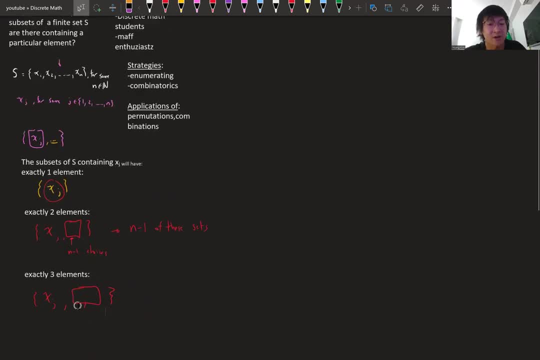 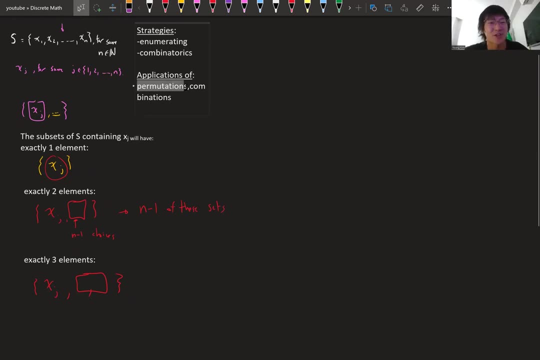 that's not this, right, so that's, then you can ask how many of these are there here. okay, so now this is the, the branch, uh, the the combinatorics branch, uh, specifically permutations and uh combinations that I want to. 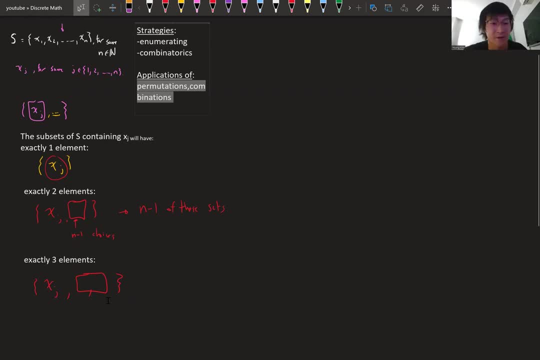 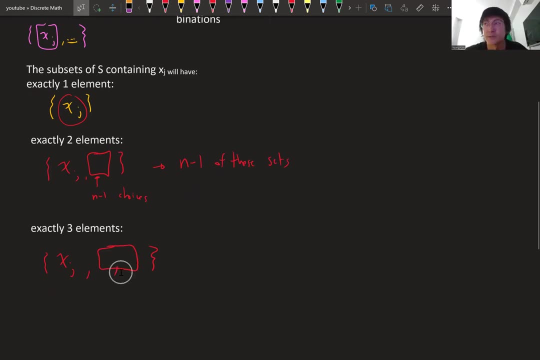 go in because you can. you can argue, you can reason about this in two ways. right, so here. so here's the first way. so the quick answer: you have to choose n. you have to choose n minus one. 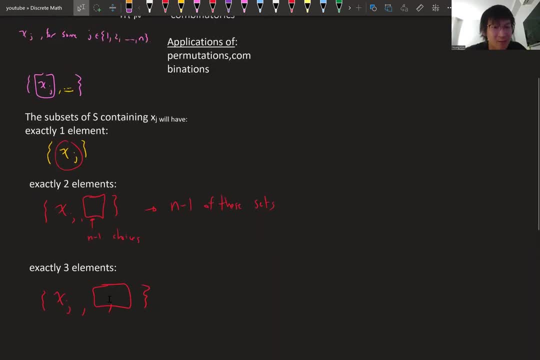 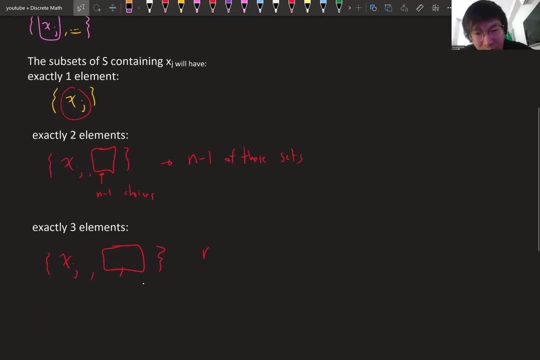 um, you have to choose two elements from n minus one things. okay, so how many choices are here then? that would just simply be n minus one, choose two. okay, once again, I'm assuming you know this stuff. okay so, but if you wanted to take the permutation, 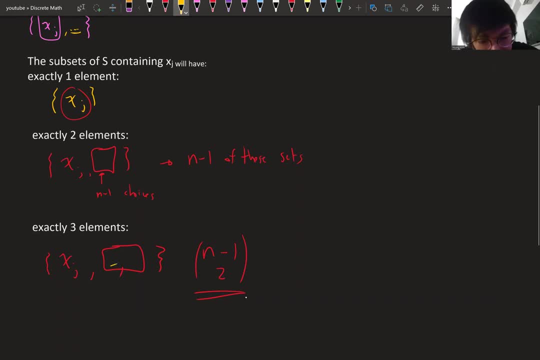 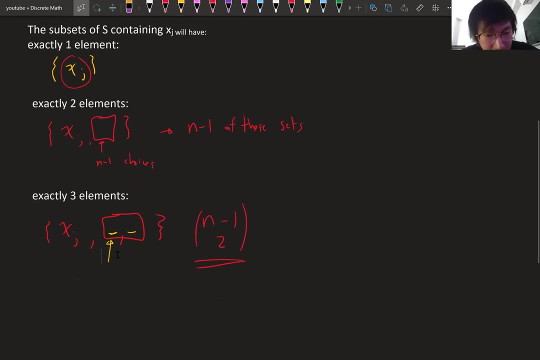 path you could. you could say: all right, first choose this and then choose this, right. so then, if you, if you want to first choose an element here for your first pick, then that would be n minus one elements and then, consequently, the second choice. you'll have one less than that. 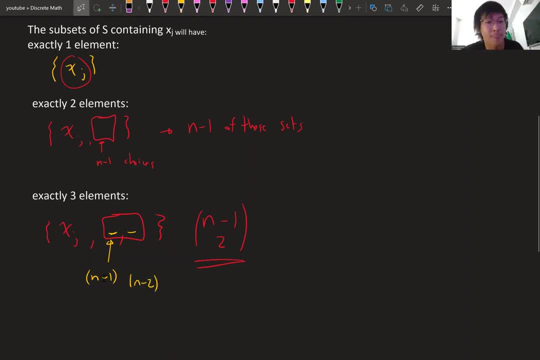 which is n minus one minus one, which would be n minus two. right, but this, this, so. so that means that, all possible, uh permutate two permutations, right, permutations of two things. it's going to be n minus one times n. 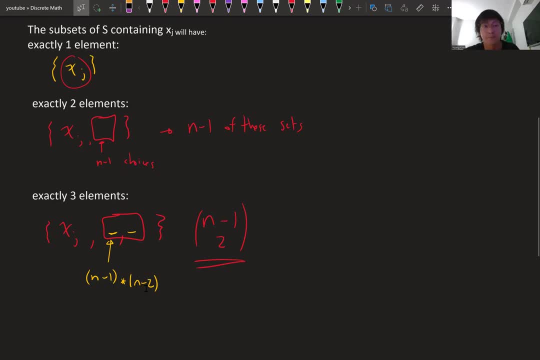 minus two by the, the fundamental countable principle. but in a set we don't care about the order here. in an ordered set, this is an unordered set. so you are, you're overcounting here by a factor of two, so you would have to divide this by two. and if you, if you actually 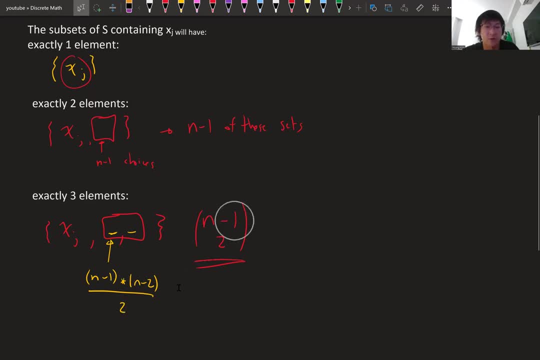 go through this, uh, this origin here, and you check this and this, that these, these are equal. okay, so, once again, this is the fastest, the faster path and this is the. this is a different path, but they both work okay. so, anyways, what was I saying? yeah, so then there are n? n minus. 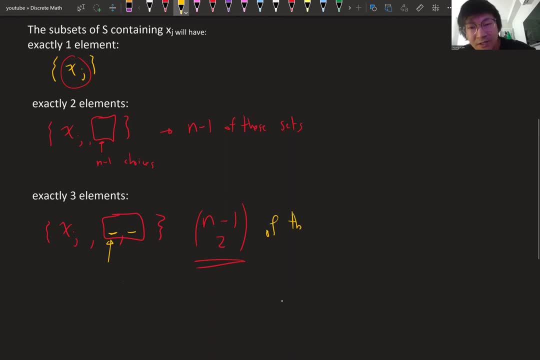 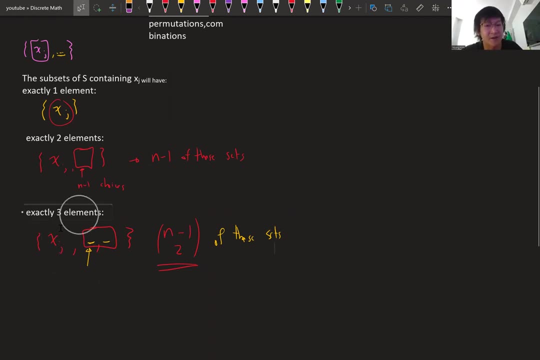 one, choose two, uh of of these of these sets, uh, that contain x of j and have exactly three elements. okay, okay. so, once again, you, so, you, you, you repeat this argument, right? and then, uh, you will stop when you hit the max, the max number of elements, right. 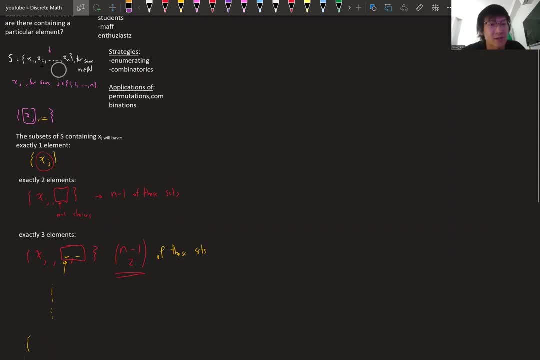 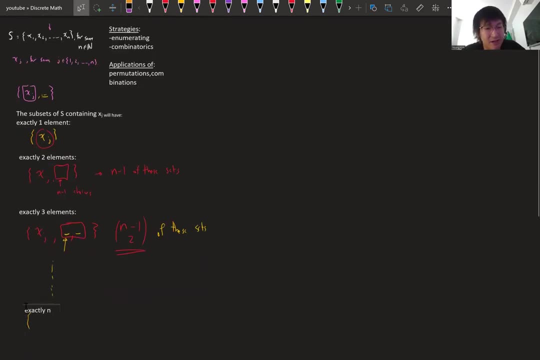 so you can include everything, right. so that's just the set s again. so this is just going to be the entire set, right? so then here you say, uh, and then the final case would be exactly n elements, right? and if you notice, uh, there's, there's, there's only one way of doing this. 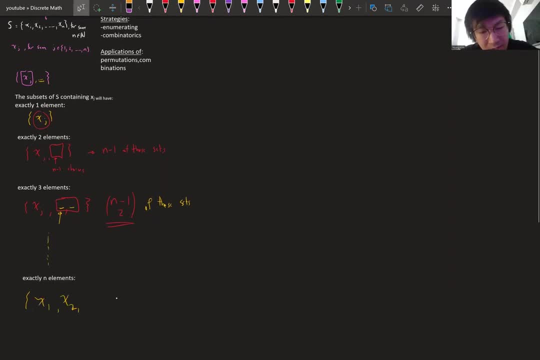 right, so it's just going to be x sub one, x sub two. uh, dot, dot, dot, dot, x sub n. okay, and um, this is also pretty cool too, because, um, if, if you uh studied a little. 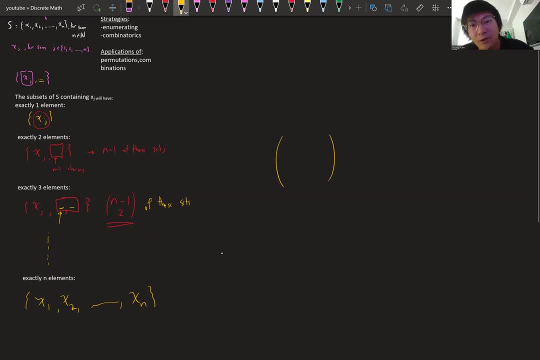 bit about uh, these, uh, what do they call these? uh, binomial coefficients, this n choose k. there's a little symmetry about this right, because if you say, like, how many things can you choose? uh, how many like, if you say, how many ways can I pick one thing from four objects? 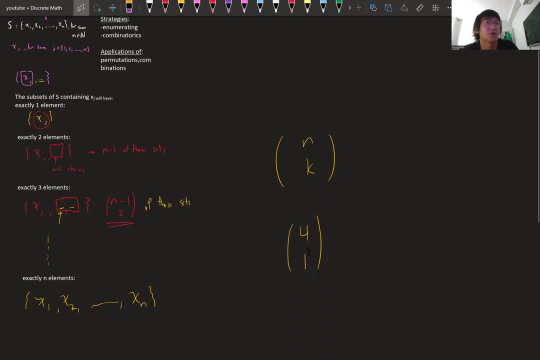 that's equivalent to uh choosing three to leave out. so then, four choose one is equal to four choose three. All right, so you could kind of, yeah, think about this and uh, when you go through this too, and you'll see it, but essentially there's only: um, there's, there's, there's one way of. 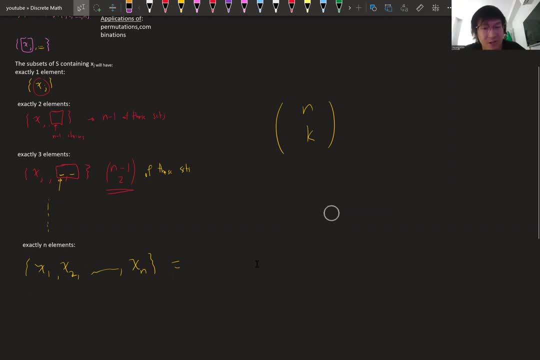 doing this right, or? or, if you want to apply what I just said here, you could just say: there are n minus one things and you have to choose exactly n minus one things from there, and this is also going to be one. okay, okay, great. so now, if you want to find the uh, all, all. 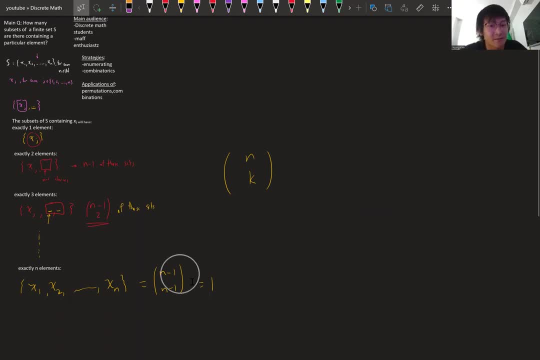 all. so the number of total subsets: right of this, you just got to add all of these. okay, you got to add all of these. how many there are? so, um, let's do that. The first choice. I didn't write it here, but if you need to, 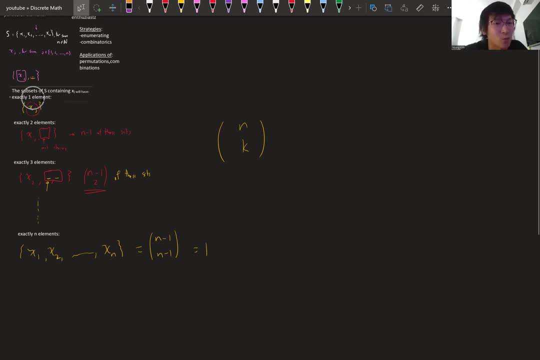 if you need to choose here with exactly one element, you have n minus one elements to choose from and you're choosing zero. so this is n minus one, choose zero, right, and then for two elements, it's going to be n minus one, choose one. 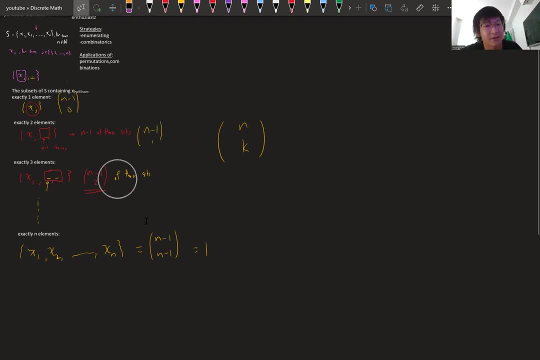 And then and so forth. so so that means that so the total number of sets of sets containing so total number of subsets of s containing x sub j- yeah, I'm just going to write x sub j because I can't type with subscripts that well. 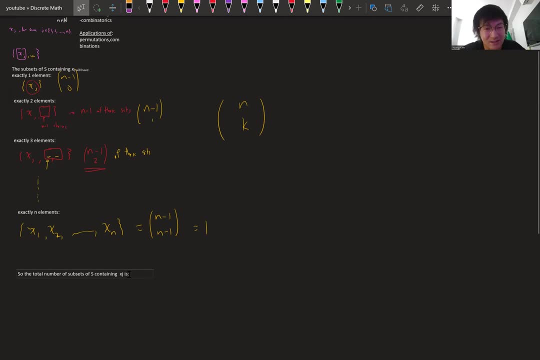 all right. so is is simply, you just add up all of these numbers, right, it's just, it's going to be n minus one- choose zero, plus n minus one- choose one plus dot, dot, dot dot. 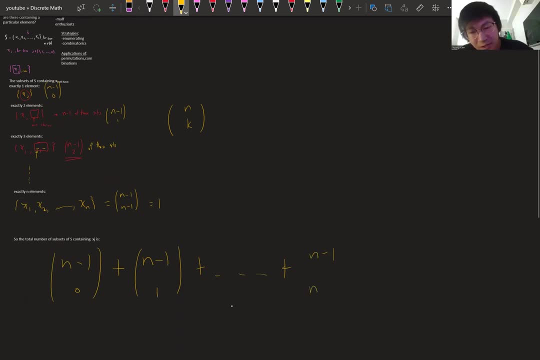 plus n minus one. choose n minus one. okay, and you could write this in closed form. if you, with your summation, and that's just going to be, that's a sigma, okay, that's a, that's a better. 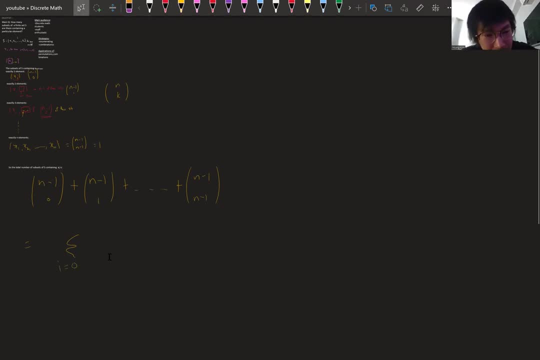 sigma, okay, here. i is equal to zero. ranges from i equals zero to n minus one. and these, these uh terms or these addends, look like uh, this form n minus one. choose i. okay, so it's it's. 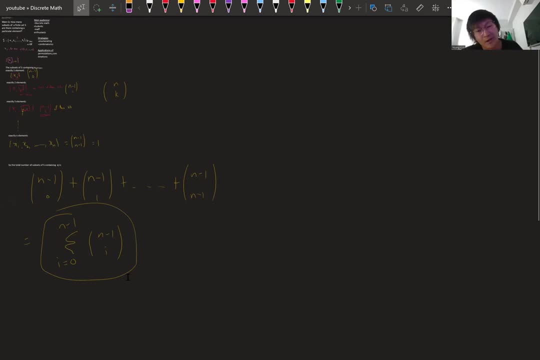 it's going to be this, okay, um, now here, this is like really, really, this is. hopefully this is not too long, but whatever, okay, so here, uh. so here, here's a more, here's a concrete. 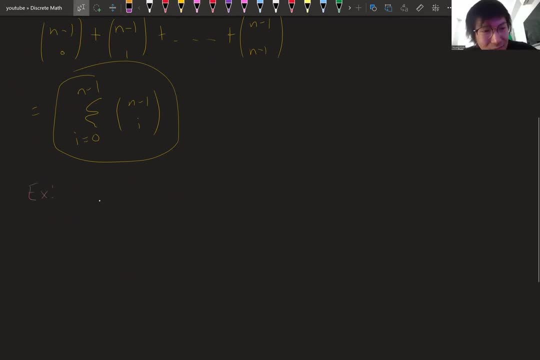 example, right? so here, example: if I gave you a set and it has these three things, first three letters of the alphabet: a, b, c, and you want to see? uh, the question is, yo, subscript typing will be the end. okay, wait, wait, give me a second. 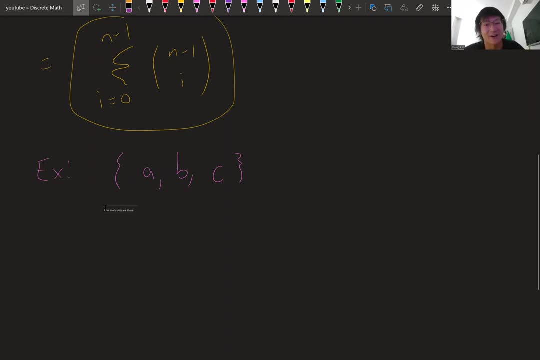 so how many sets, how many subsets are there? uh, containing b? okay, uh, let me call this set s and s. all right, so then here you just got to see the number of elements there are, right. so here there's three, and you could just plug it into this formula. 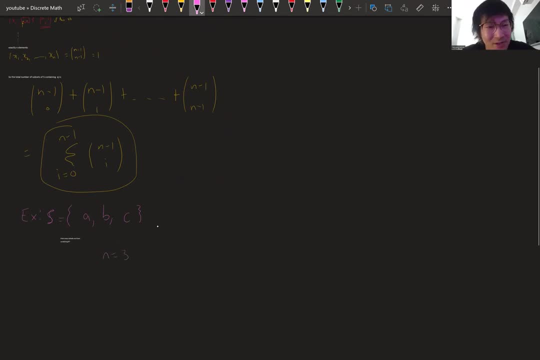 right. so then here n is equal to three, which implies n minus one is equal to two, and then you plug and chug, I'll just plug. so i i equals zero and uh, this is going to be two. 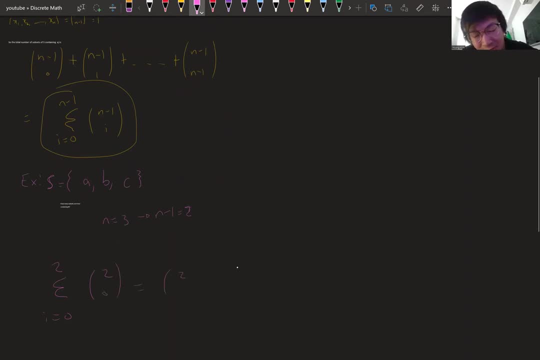 and you're going to say two choose zero. sum that up, so it's two choose zero plus two choose one plus uh, two choose two. and we said earlier that this is one one and this is two, so there's. 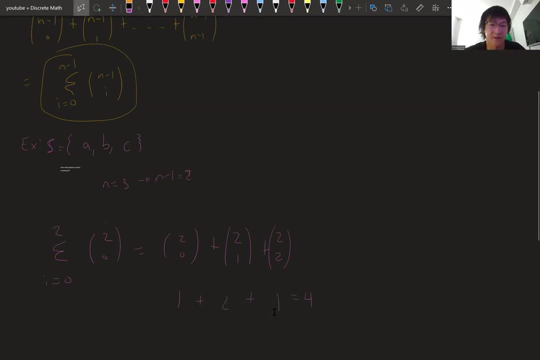 going to be: uh, four, four, four elements. okay, so, once again, um, you could use this formula, right, but this is not going to tell you exactly how the the subsets will look, but it will give you the count. okay, now, if you want to actually see, uh, these subsets. 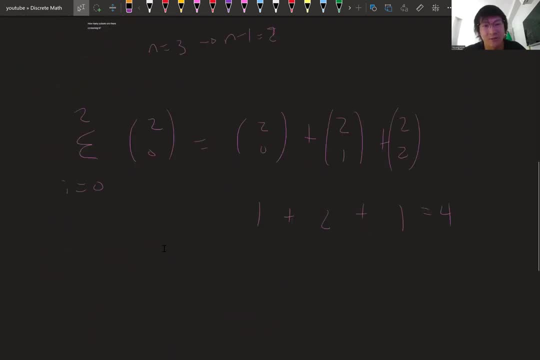 then you would, uh, yeah, use some kind of enumeration, um, um, enumeration thing and trick, and we could do that here, right, uh, um, so here. so let me show you so here: how many sets are there containing? okay? 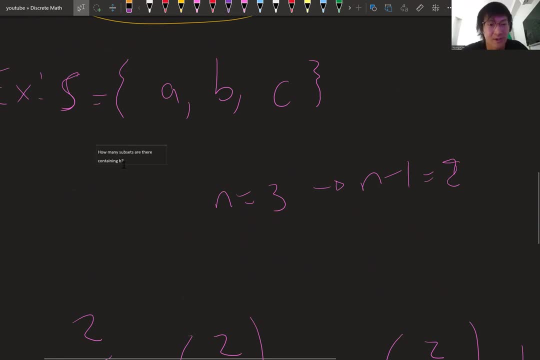 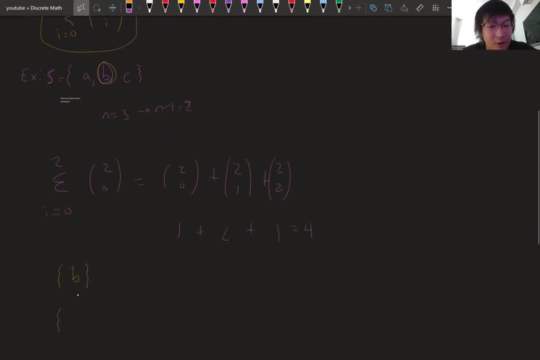 to be in the second. that's it, that's the singleton, right, then you could take b and depend. uh, you have two choices, right. so then that's. you could say b comma a, and then you could also say b comma c. okay, so this is the case where just one element would be. 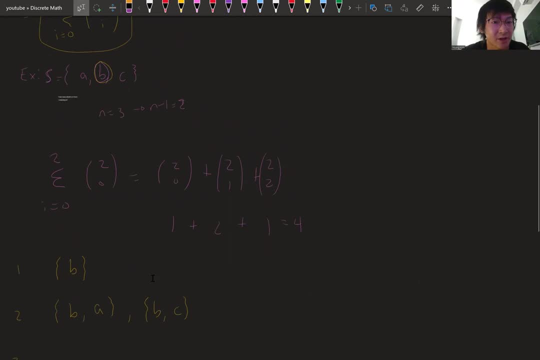 and two, two elements would be, and this is three elements would be, and then you only have exactly one choice, which is just to set s again, okay, and if you count these, you get one, two, three, four, and this is this. this, this checks out. okay, now there is a more systematic way of doing. 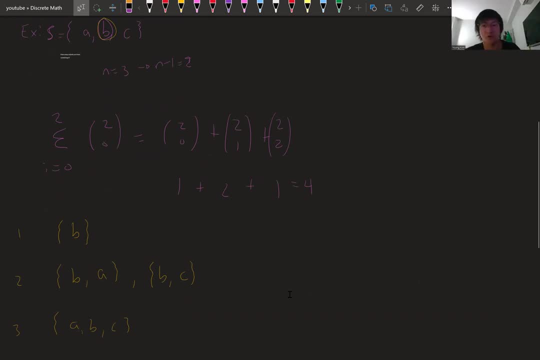 this and um uh, you could kind of like create a table and convert this into like a weird uh bit problem, so let me just show you. so, um uh, let me look at my notes. I forget. 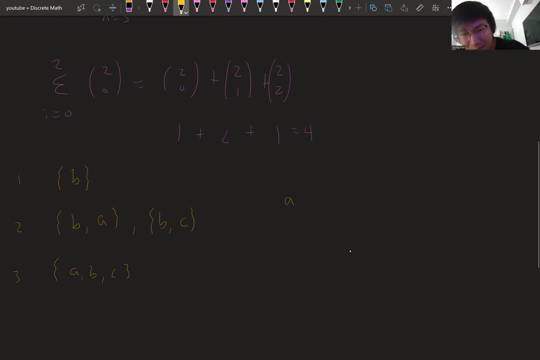 okay. so here you, you write the elements of this set that you're given- a, b, c, like this right, and we said that you, uh, you, you, you necessarily want to include this. okay. so, um, in this table, what you can do is use two symbols. oftentimes they use one and zero. 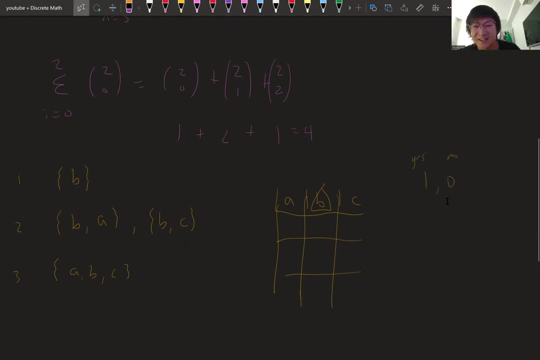 for yes, that's in the set, and no, for that's not in the set. right, um? or you could use a check and an x doesn't really matter, smiley face, poop, emoji, whatever, right? so here, um, if, if we so, let me use the check. right? so, if, if I'm? 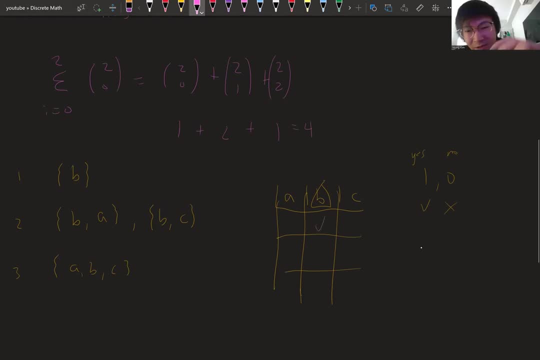 saying that this is this has to be in it, then that means that you, you check this and then you can. you can go, you can go through these, right, do I include a? then you could say, uh, uh, yes.